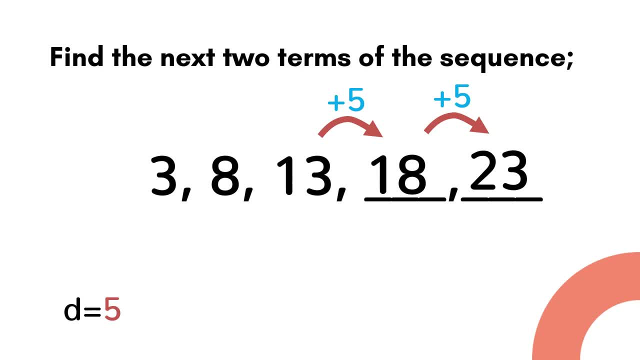 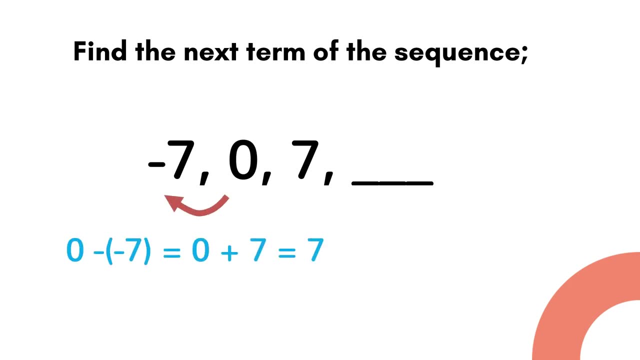 Therefore, the next two terms of the sequence are 18 and 23.. Now let's discuss the last example. Find the next term of the sequence: negative 7, 0, 7.. The common difference, that is 0 minus negative 7, is equal to positive 7.. Take note that if the 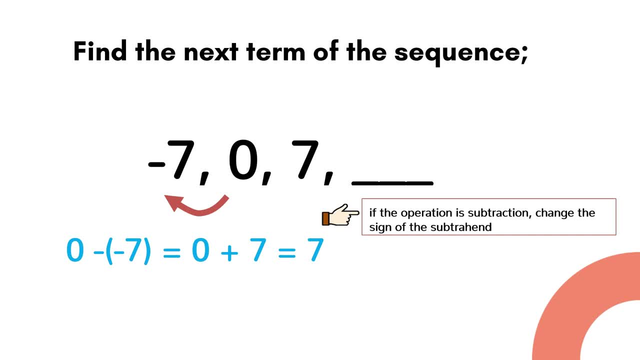 operation is subtraction. you have to change the sign of the subtrahend, So the common difference is equal to 7.. Then we just add 7 to the last term, given that is, 7 plus 7 is equal to 14.. 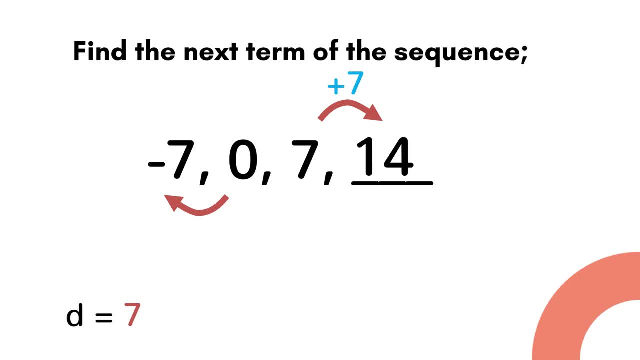 Thus, the next term of the given sequence is 14.. That's all for today. Thank you for watching. I hope you learned something.